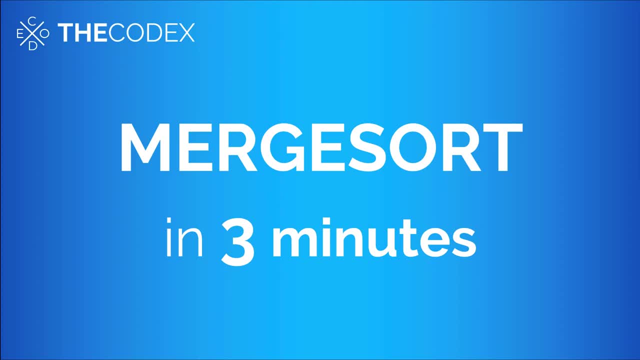 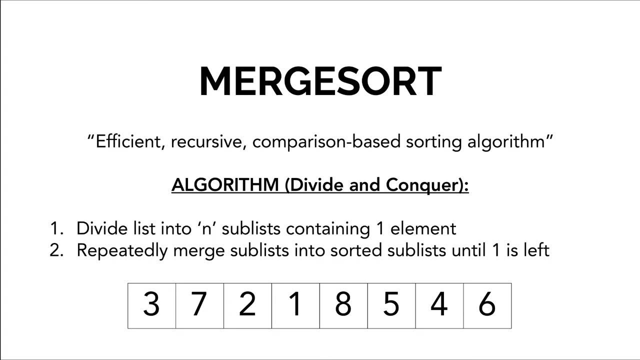 Hey guys, my name is Avi and I'm from the Codex, and today we're going to learn MergeSort in 3 minutes. Now, what is MergeSort? MergeSort is a computer science algorithm that uses recursion to go ahead and sort any list or series of data you give it. The algorithm it uses is called Divide and 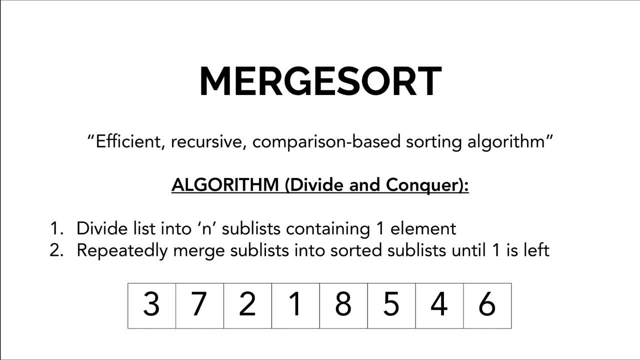 Conquer. What it does is it's going to go ahead and take your array, no matter how big it is, and continuously divide it until you have n number of one element arrays. For example, in our case we have 3,, 7,, 2,, 1,, 8,, 5,, 4, 6.. MergeSort would go ahead and create 8 separate. 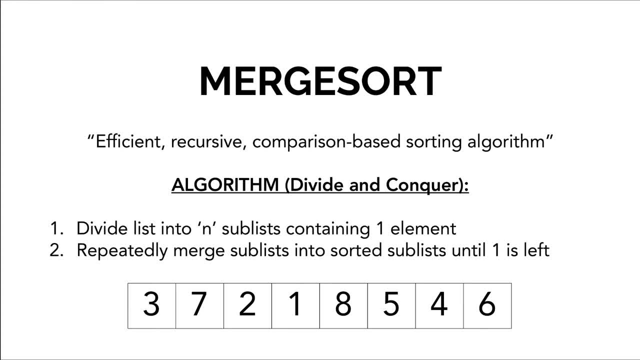 arrays that are one item big. After that, guys, once you have a bunch of one element arrays, you're going to go ahead and merge those arrays, creating 2, then 4, then 8, until you've completely sorted all of your different items and you have one giant array that's completely sorted. That's. 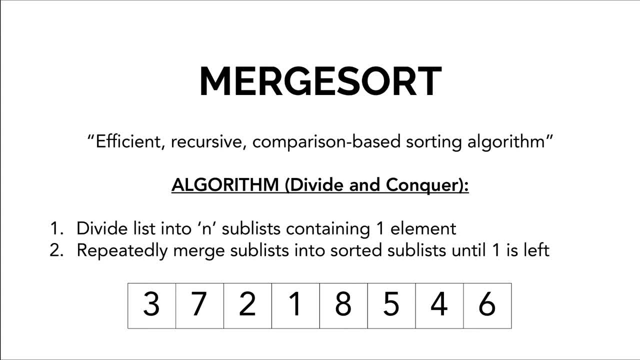 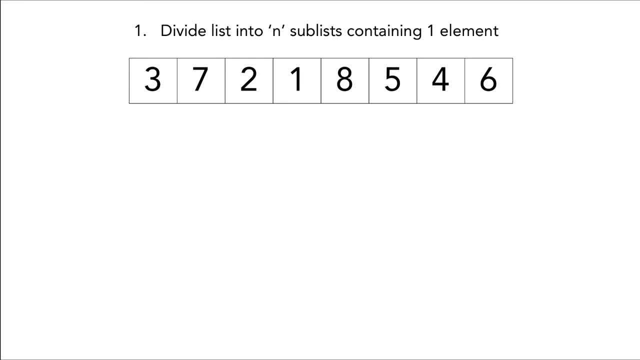 exactly how MergeSort works. Let's go ahead and see a live example in this tutorial Over here. we have an array: 3, 7, 2, 1, 8, 5, 4, 6.. MergeSort, again, is to go ahead and divide it into n sublists containing one element. 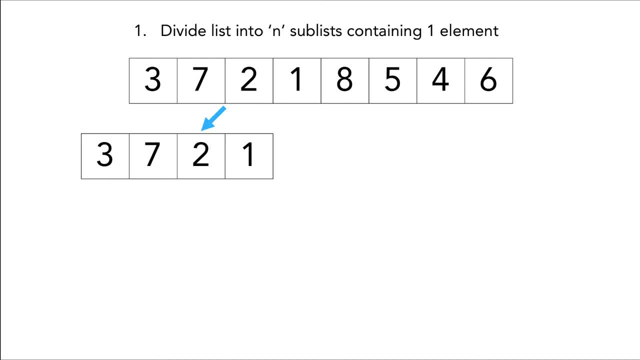 So what we're going to do, guys, is we're going to take our array and split it in half: 3, 7, 2, 1, 8, 5, 4, 6.. Then we're going to take the two newly created arrays and split them in. 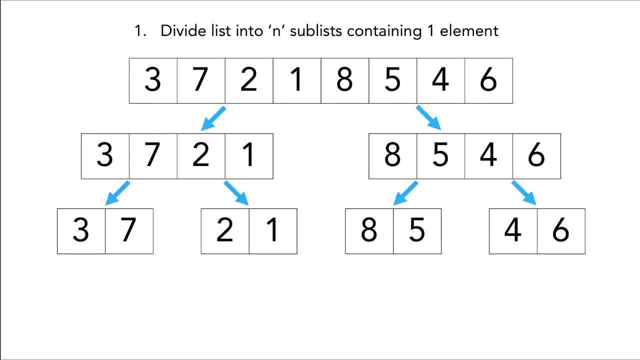 half again: 3,, 7,, 2,, 1,, 8,, 5,, 4,, 6.. Last but not least, guys, we're going to take the arrays we just created and split them in half again: 3,, 7,, 2,, 1,, 8,, 5,, 4,, 6, until we have n sublists. 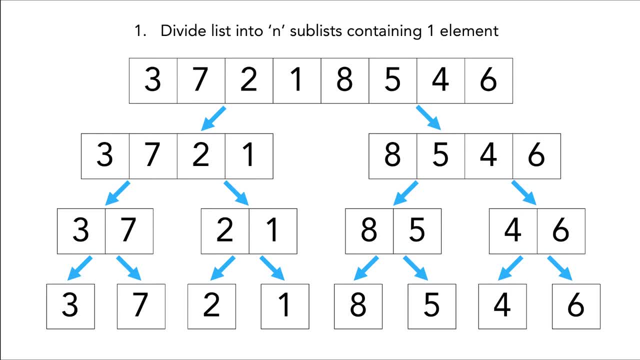 containing one element. Now again, guys, MergeSort is based off of recursion. So, theoretically, what would happen is due to recursion. recursion would take our first array, break it in half. but instead of breaking this in half again, it's going to focus on this array and completely break it in half. So it's going to. 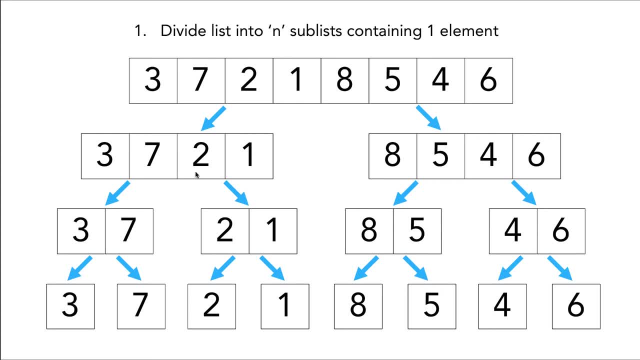 say 3,, 7,, 2,, 1, then go down this path over here. then take the other side of 3,, 7,, 2,, 1,, go down over here, et cetera. Recursion is a little bit more complicated but to make MergeSort easy to 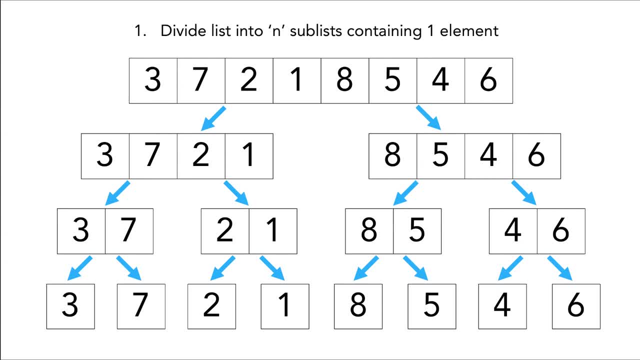 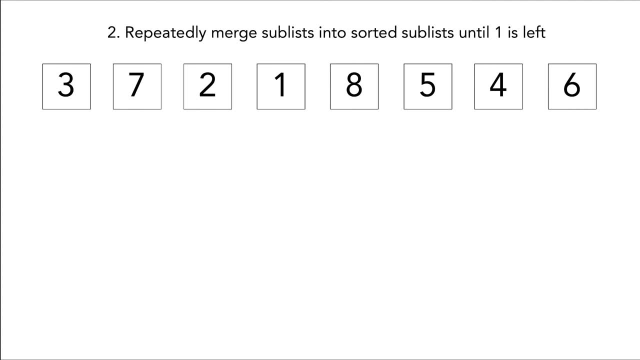 understand I'm showing all of the processes at once. All right, so now we have our eight single item array, Let's go ahead and take a look at the next step: repeatedly merge sublists into sorted sublists until one is left. So now that we have eight items or eight arrays, we're going. 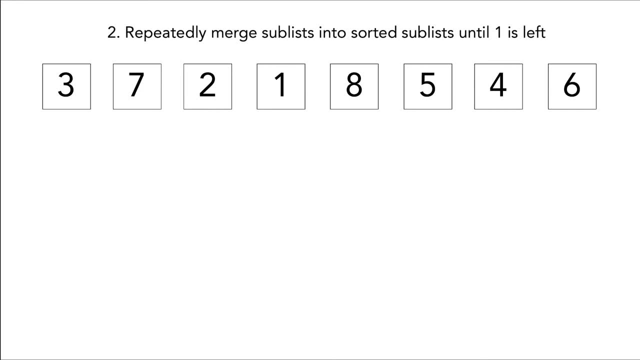 to go ahead and merge them back into one big array, except now we're going to sort them. So here we have 3 and 7.. 3 and 7 is in the right order. So when we create an array, we're. 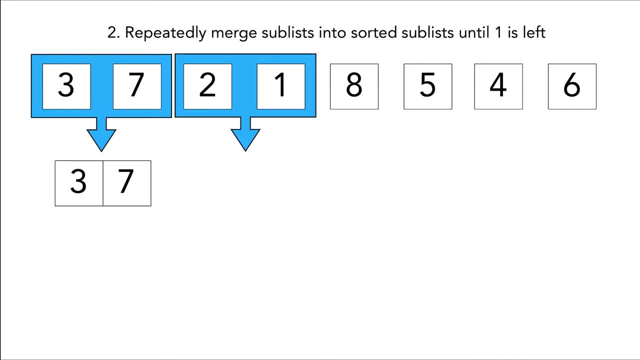 not going to change anything. Our next step is 2, 1.. However, we know that 2 is greater than 1, so we're going to say 1, 2.. We know that 5 is greater than 8, so we're going to. 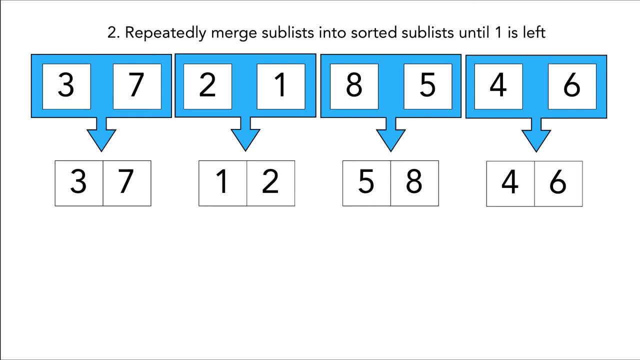 say 5, 8, and then 6 is greater than 4, so that stays the same. Now, with our newly created arrays, we're going to merge these two and these two. So we're going to go ahead and say 1,, 2,, 3,, 7,, 4,, 5,, 6,, 8.. And then, last but not least, we're going 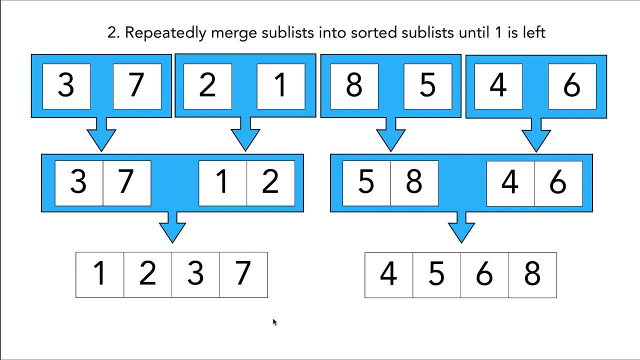 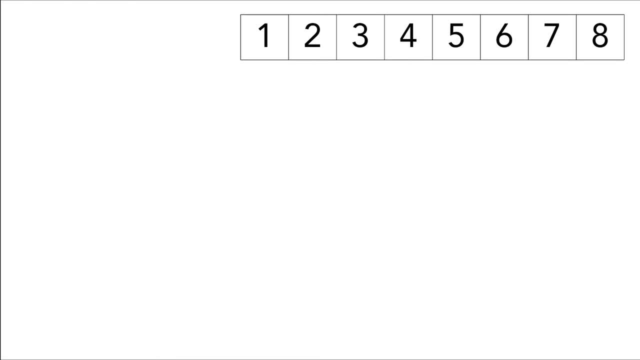 to merge our two four-item arrays into one massive eight-item array. that will be sorted and we get over here: 1,, 2,, 3,, 4,, 5, 6, 7, 8.. Fantastic, MergeSort has a big O of O N log. 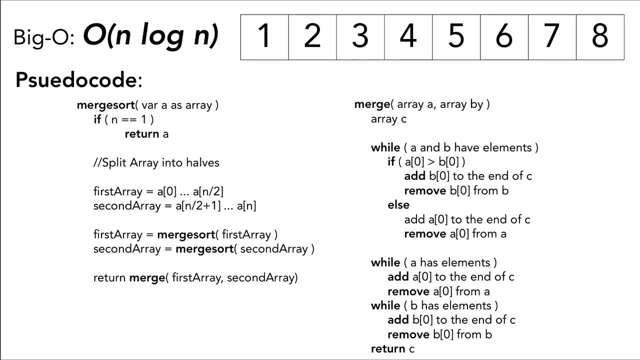 N and here is the pseudocode, if you need Again. it consists of two functions: MergeSort and Merge. MergeSort is a big O of O N log N, and here is the pseudocode, if you need Again. it consists: 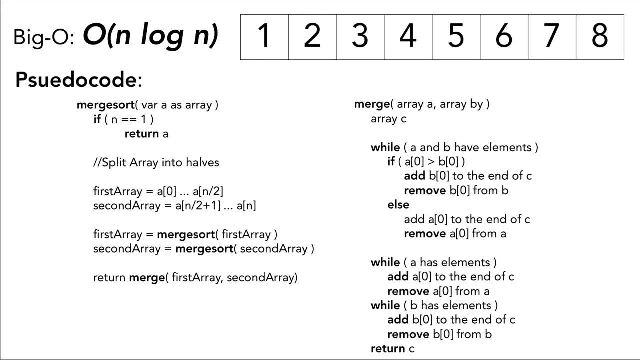 of two functions: MergeSort and Merge. The MergeSort function is what you actually run with the array. It will go ahead and split the array into halves until you have single-item arrays and then, once you have single-item arrays, it's going to go ahead. 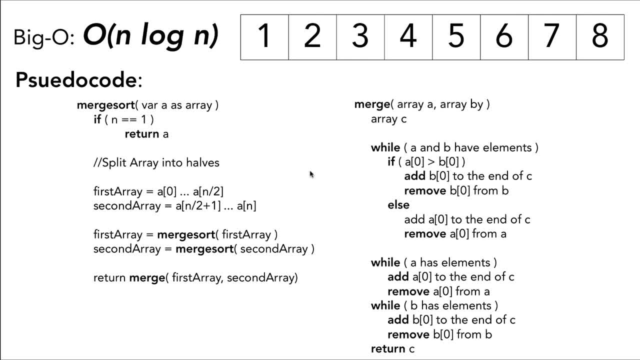 and run the Merge function. The Merge function will go ahead and join those elements together until you create your final array, which is sorted and looks just like this above. Thanks so much for listening, guys. That was MergeSort in a nutshell. If you have any questions, 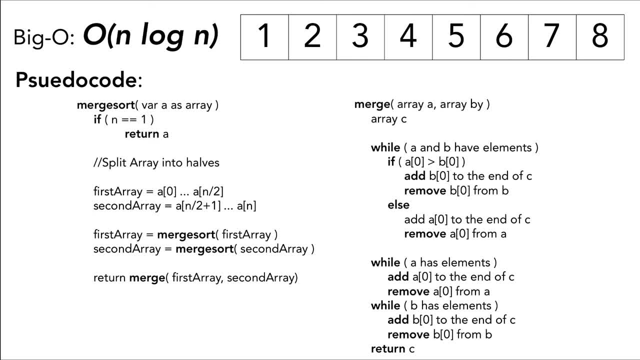 let me know. Don't forget to like, share and subscribe, and I will see you in the next video. Bye-bye. 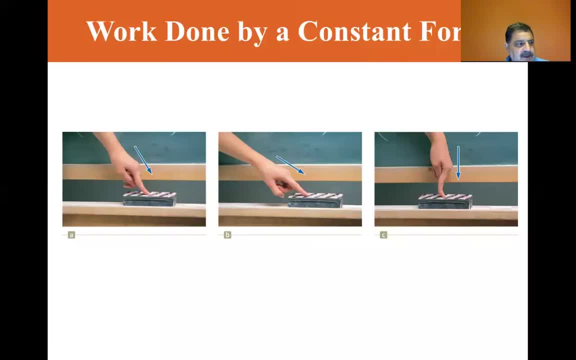 Okay, we're starting section 7.2, work done by a constant force. Now there are many mechanisms by which a system can be influenced by its environment, And the first one we're going to look at is work. Now the meaning. we use the word work every day, but the physics meaning